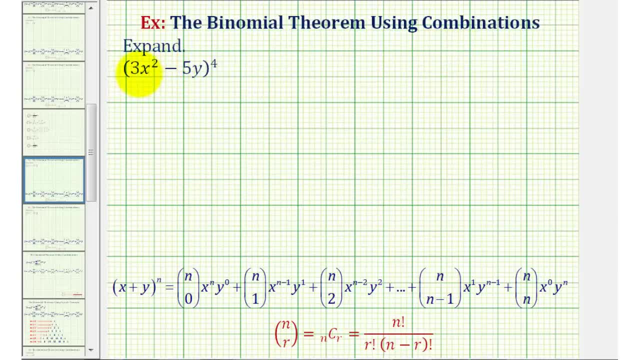 We want to use the Binomial Theorem to expand the quantity three x squared minus five y raised to the fourth power. The Binomial Theorem is stated here below, and while it does look fairly involved if we break each term down into three parts. 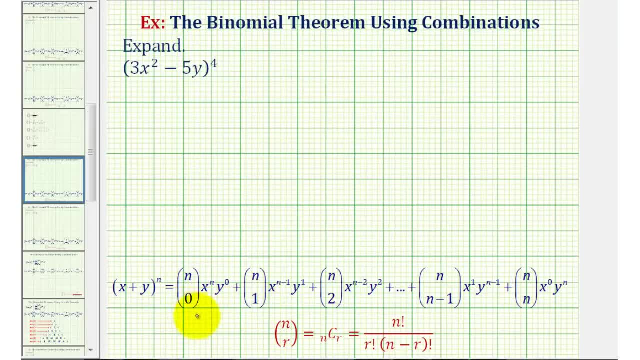 we'll be able to see the pattern, which will make this much easier to remember. So, if we have the quantity x plus y raised to the power of n, notice that each term has a factor, that's a combination. It has a factor from the first term, x, and has a factor from the second term, y. 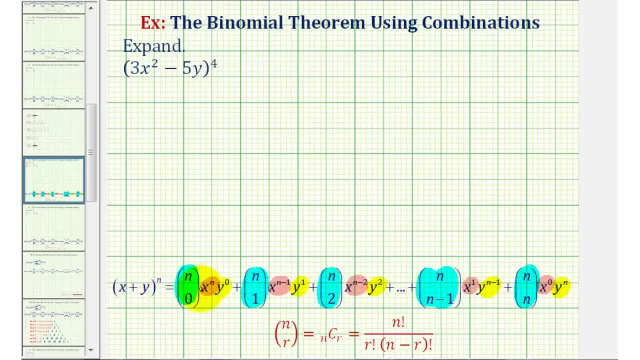 If we look at just the combination factor, notice how the first combination is n choose zero, where n is the exponent on the binomial. The next term has n choose one, followed by n choose two. This pattern continues out to n choose n. 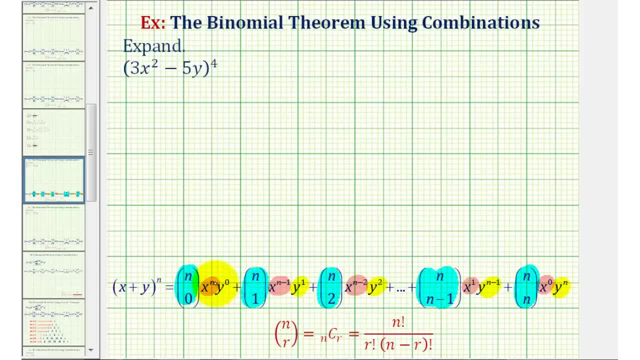 Looking at the factors of x and y, notice how the first term contains x to the power of n, where n is the exponent on the original binomial and we have zero factors of y. And then for successive terms, we drop one factor of x and pick up one factor of y. 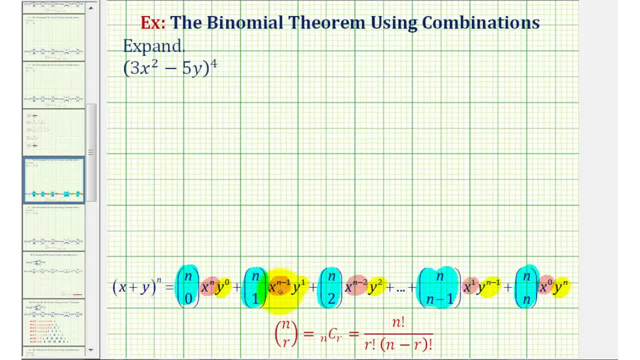 Notice: the next term has x to the power of n minus one and y to the first. The next term has x to the power of n minus two, y to the second, and so on until we have x to the power of zero and y to the second. 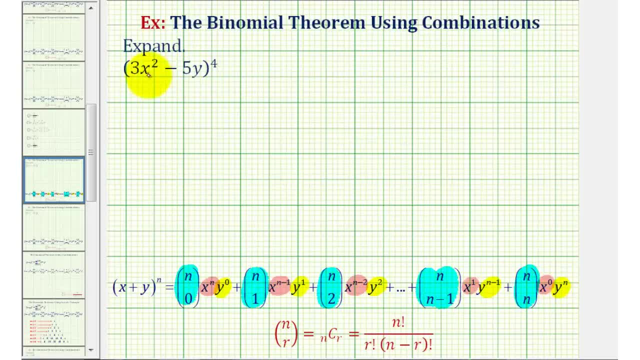 And then we have y to the power of n. So to expand the quantity three x squared, minus five y raised to the fourth power, the first term will have a combination of four choose zero. And then, because the first term is three x squared, we'll have four factors of three x squared. 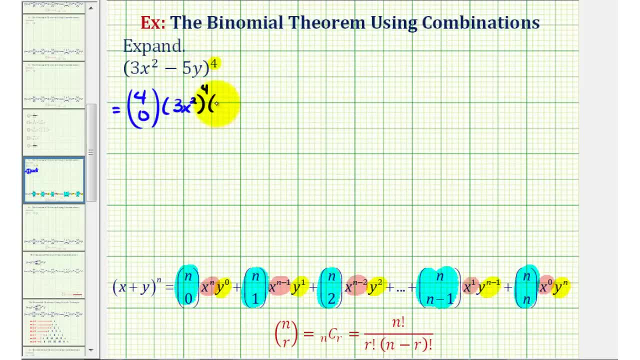 And because the second term would be negative five y, we have zero factors of negative five y. So we have the first term in the expansion, plus the next term will have a combination. four choose one, And now we're going to lose one factor of three x squared, so we'll have three x squared to the third. 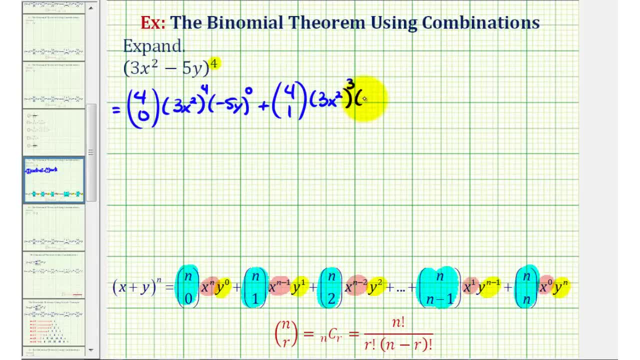 And we start picking up factors of negative five y. So we have negative five y to the first, plus next term, we'll have four, choose two. And we'll have two factors of three x squared and three factors of negative five y. For the next term, we'll have four, choose three. 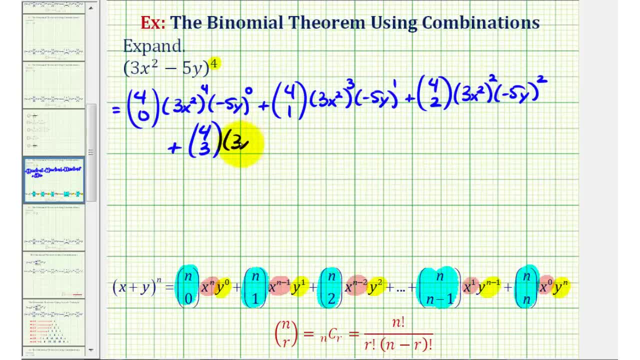 And we'll have just one factor of three x squared and three factors of negative five y. We have one more term. We'll have four. choose four times zero factors of three x squared and four factors of negative five y. Now we've applied the binomial theorem. we just need to simplify this. 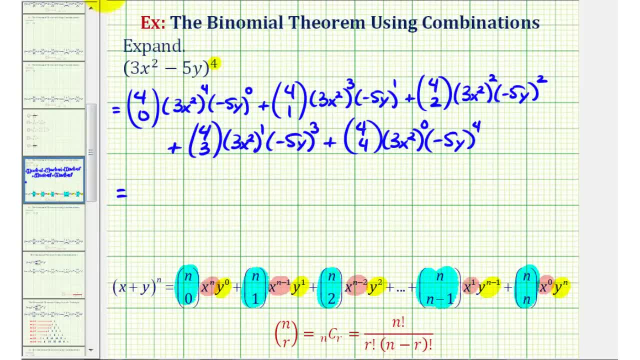 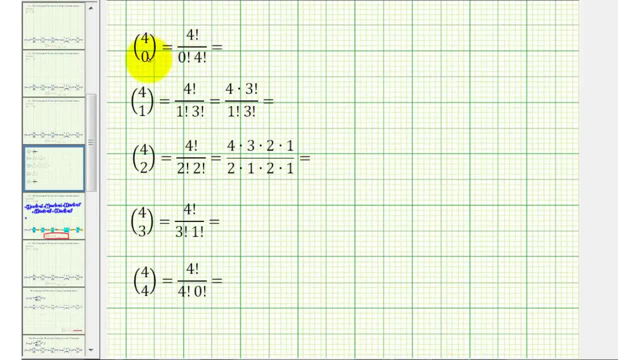 So for this first term we have four choose zero. We're using our definition here for a combination: Four choose zero is equal to four factorial divided by zero factorial, four times four factorial. We can see this simplifies nicely to one. And zero factorial is equal to one, so this simplifies to one. 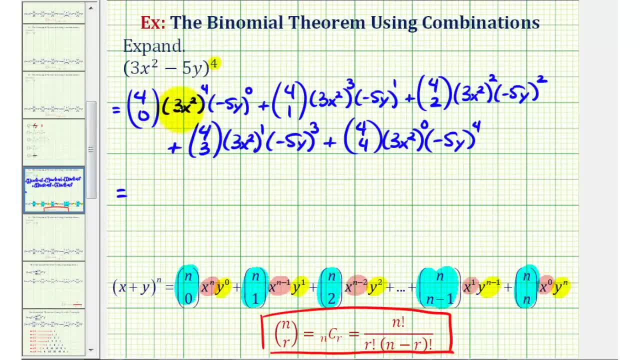 So for this first term, we would have one times three: x to the second raised to the fourth. Well, three to the fourth is equal to eighty-one, X to the second raised to the fourth is x to the eighth, And then negative five, y to the zero, power is equal to one. 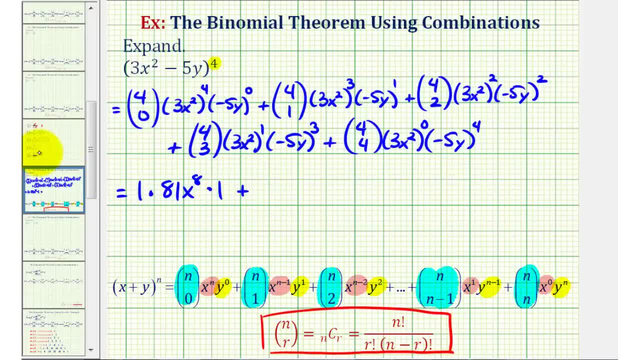 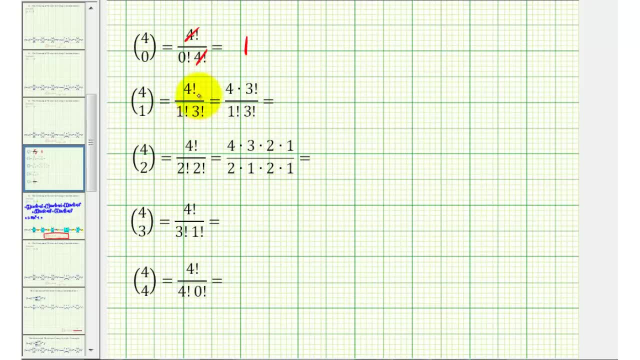 Plus we have four choose one. let's go look at that. Four choose one is equal to four factorial divided by one factorial times three factorial. But we can write four factorial as four times three factorial In this form: notice the three factorial over three factorial simplifies to one. 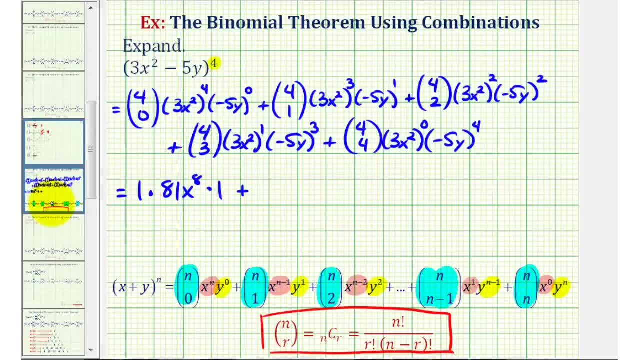 So this simplifies nicely to four, Which means for the second term we'll have four times three to the third is twenty-seven, X to the second to the third is x to the sixth, And then we have one factor of negative, five y. 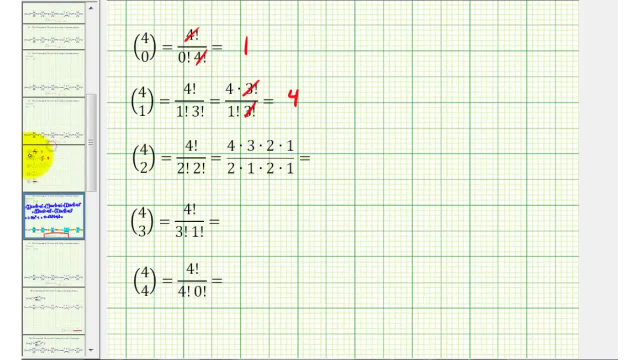 Plus four choose two. Let's go look at that: Four choose two is equal to four factorial divided by two factorial times two factorial. So if we expand these it would look like this: Notice: two times two is equal to four. So four over four simplifies to one. 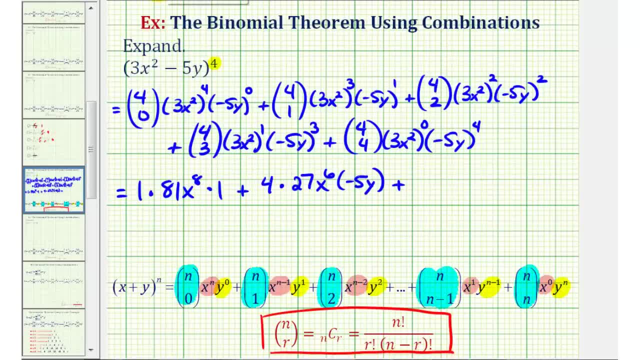 This simplifies nicely to six. So the third term is going to be six times three: x to the second squared. Well, three squared is nine. X to the second squared is x to the fourth, And for negative five y squared, that would be twenty-five y squared. 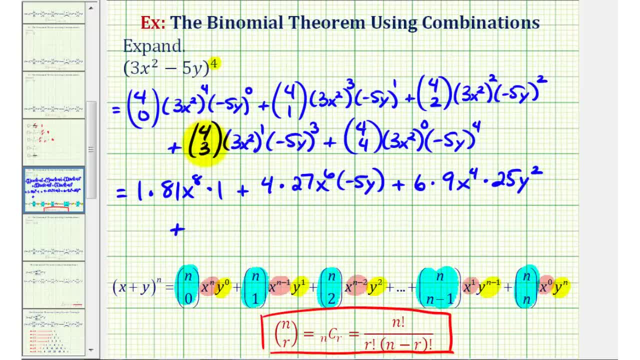 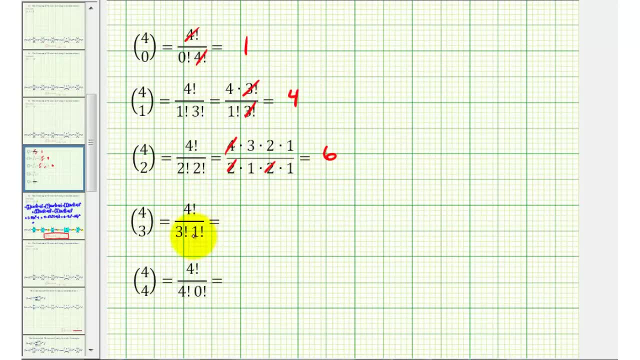 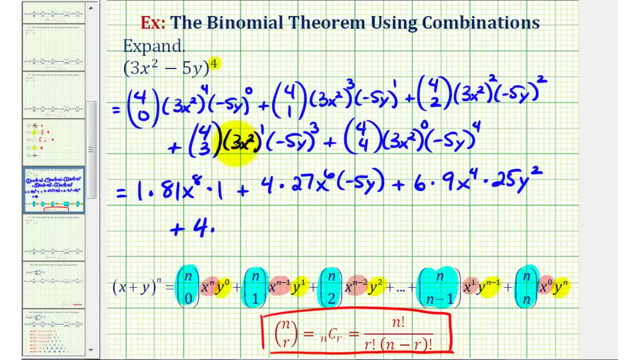 Now for the fourth term. we'll start by evaluating four choose three. Well, four choose three is equal to four factorial divided by three factorial times one factorial. Notice: this fraction here is equivalent to this fraction here. Therefore this simplifies to four. So we have four times one factor of three x squared. 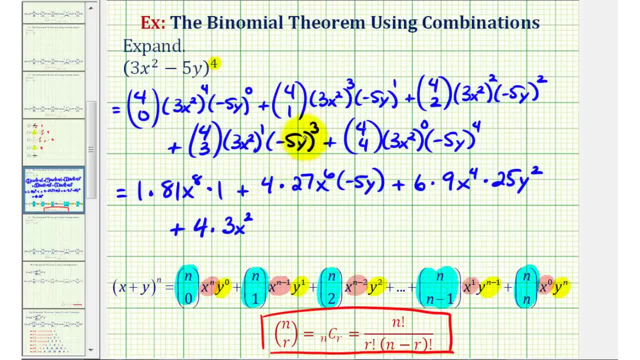 And then negative five, y to the third. Negative five to the third is equal to negative one hundred twenty-five. Then we have y to the third. Now for the last term, we have four choose four. Four choose four is equal to four factorial divided by. 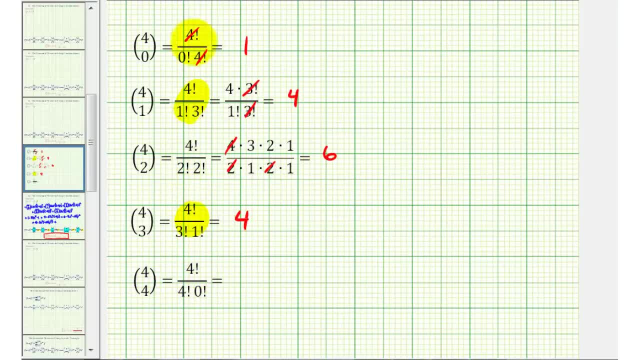 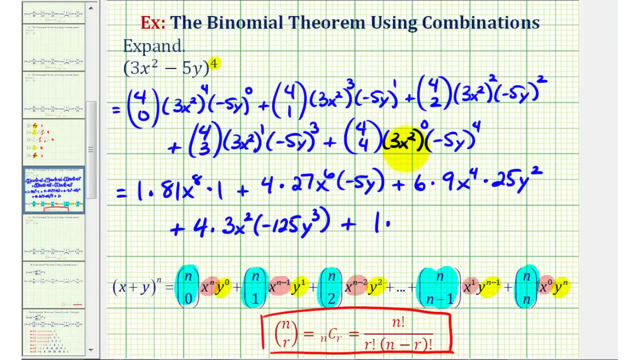 four factorial times, zero factorial. Notice how this fraction here is equivalent to this fraction here. Either way we can see this simplifies nicely to one. So our last term is going to be one times three x squared to the zero, power is equal to one. 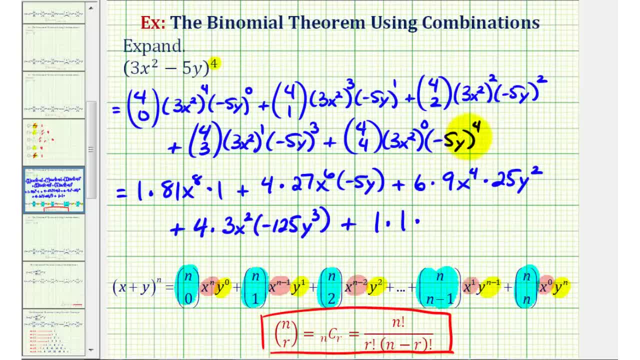 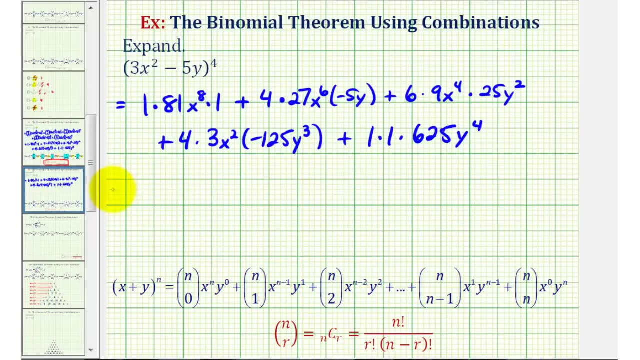 times negative five y to the fourth. Well, negative five to the fourth would be positive six hundred twenty-five. And we also have four factors of y. We'll simplify this one more time on the next slide. So for the first term we just have eighty-one x to the eighth. 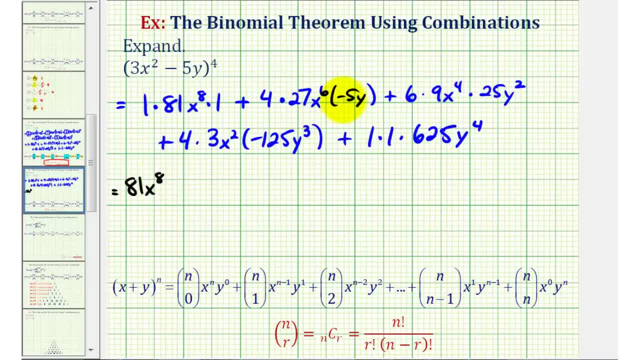 The next term. we have four times twenty-seven times negative five, That's equal to negative five hundred forty. And then we have x to the sixth y, So we'll have minus five hundred forty, x to the sixth y For the next term. we have nine times six times twenty-five.